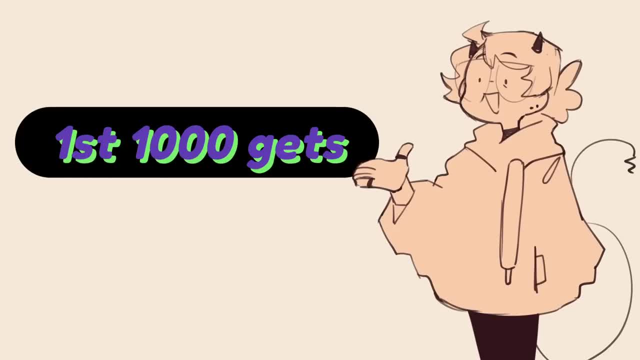 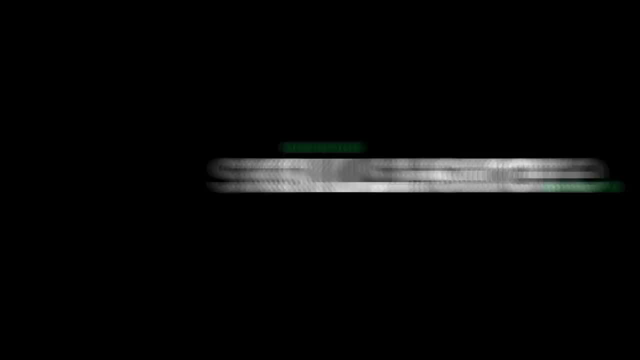 a future career. If you're interested in joining Skillshare, the first 1000 people to join the link in my description will get one month free. Thank you again to Skillshare. and now onto the video Perspective. Perspective is something I recently started drawing. I felt like I needed to add something. 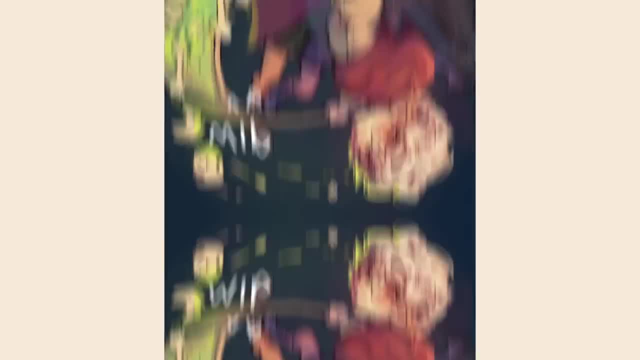 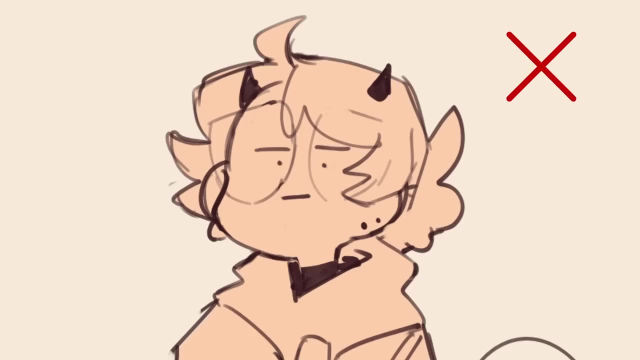 to the spice of my character art and make my pieces look more interesting. I was stuck putting my characters in the same perspective over and over again and I really dislike drawing feet and legs, so there was no way I was going to draw full bodies through the spice of my art. 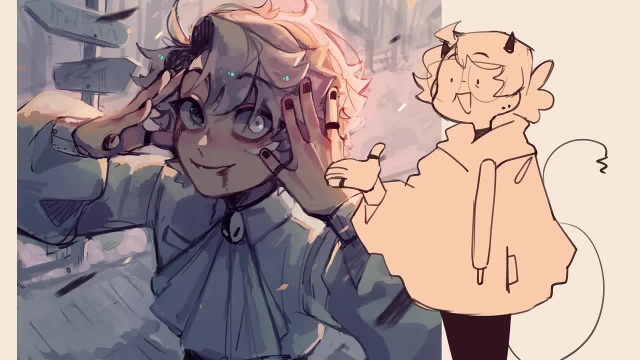 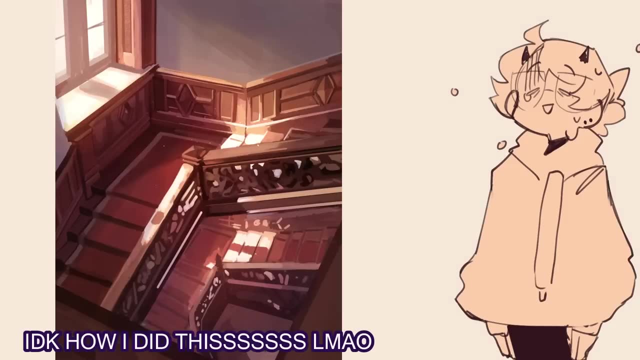 So, to make things a little bit more interesting, I started adding perspective, and I'll show you how to do that. Backgrounds, along with environments, aren't something I've put a lot of time to learn in perspective, so instead I'll be showing you how to draw perspective with like character art. 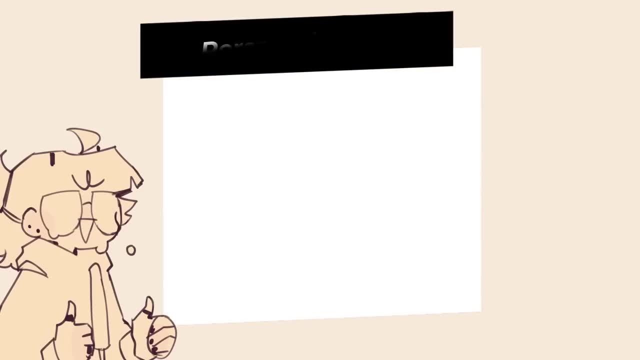 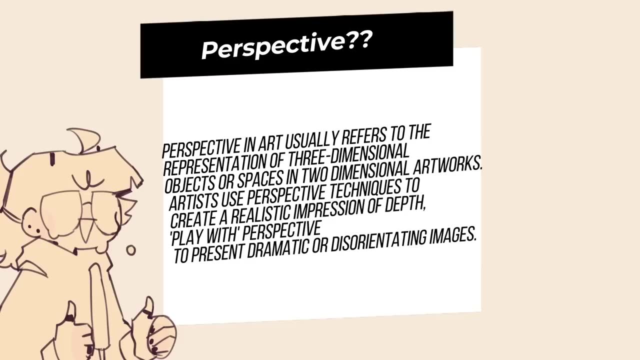 First, what is perspective? As Google defines it, perspective in art usually refers to representation of three-dimensional objects or spaces in two-dimensional artworks. Artists use perspective techniques to create realistic impressions of depth and to play with perspective to present dramatic or disorientated images. 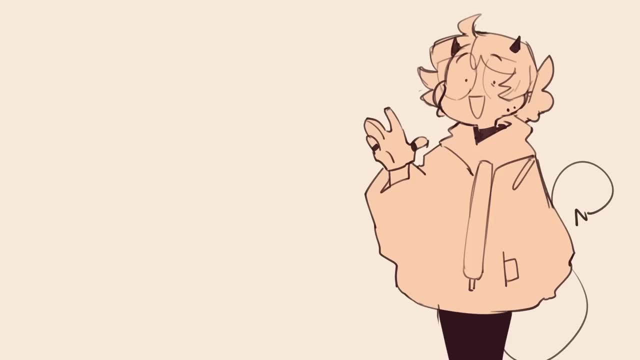 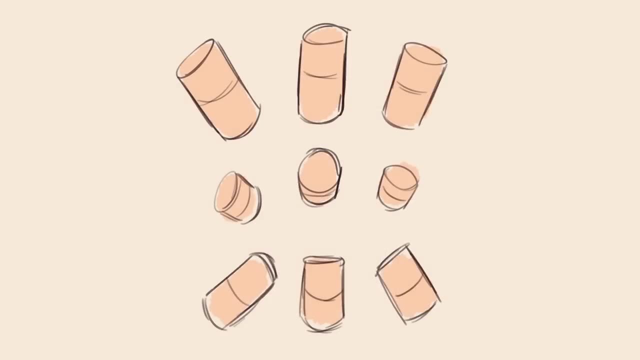 So, now that we know what perspective is, let's get down to the basics. Knowing about your perspective, it's important to be able to draw perspective Shape, as in form. so to make sure you know a little bit about form to be able to get used to this. I have a video about covering the basics. 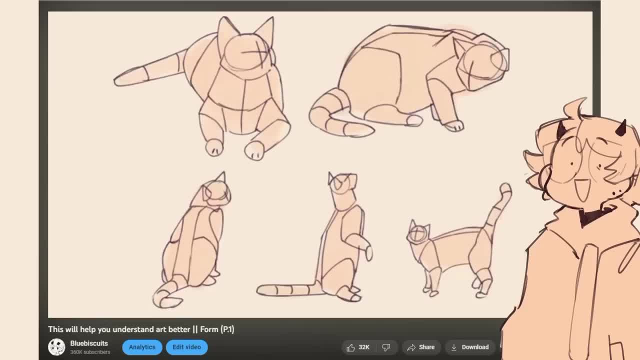 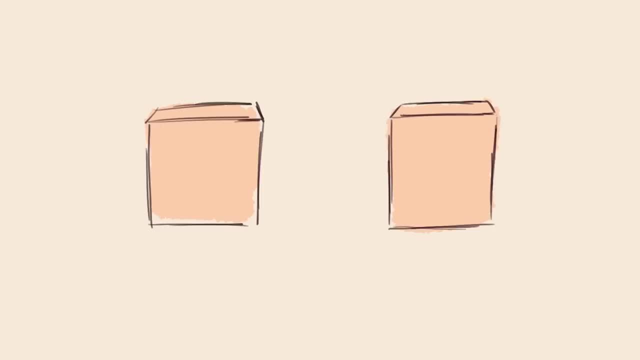 of how to draw form and how to learn it and why it is important, and I'll have that linked in the description. Here's how shape can come in handy. When you're drawing perspective, you're taking shapes and adding one closer to the viewer and one further, or you're stacking them on top of each. 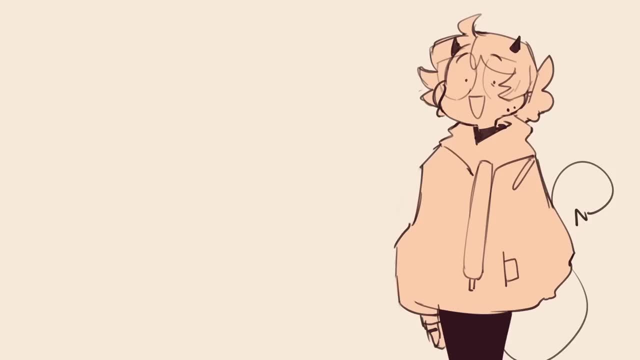 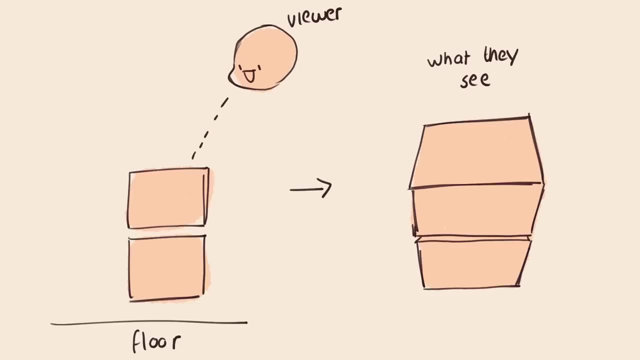 other. Now, these are just shapes, but I'll show you how I use this method to draw this with an anatomy. The important part is knowing how far the viewer is from the floor or shape and what angle is it. To determine this first, you can make a small diagram to the side, where 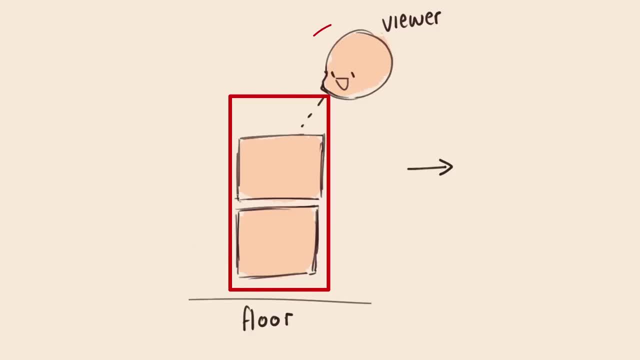 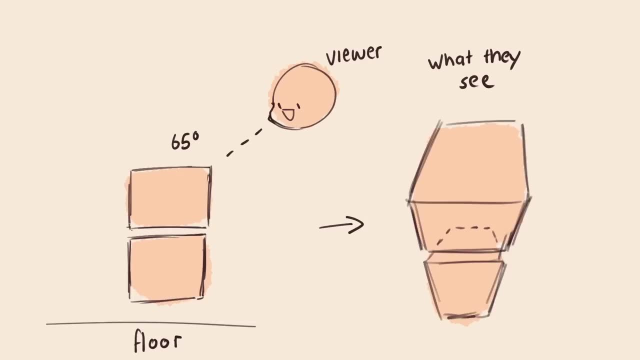 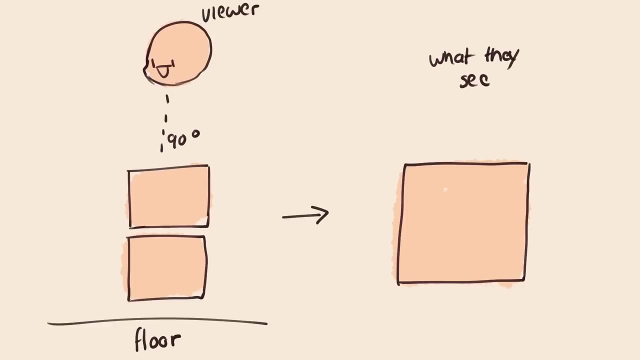 the floor is and where the shape is and where the viewer is. It's kind of like a planned out camera sequence, I guess you can call it. The angle is also very important. so, like from a 60 degree angle, the shapes will look like this. from 85 they look like this 90 and 130.. So just like. 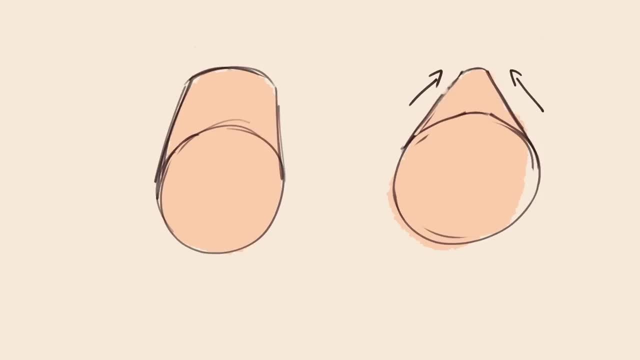 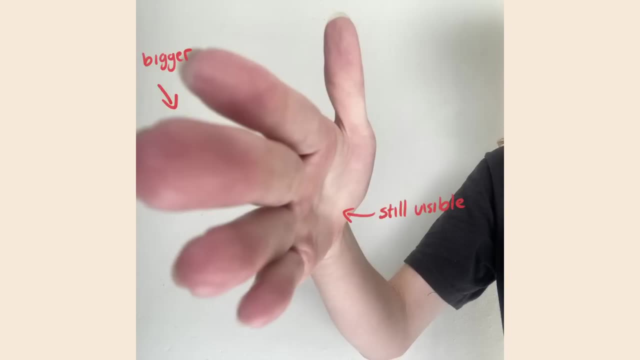 from which angle that the viewer is looking at. You can dramatically design the shapes in the background a lot smaller than the ones in the front. This depends on how close the object is to the viewer. like this, My finger is obviously bigger than my palm, as my hand is. 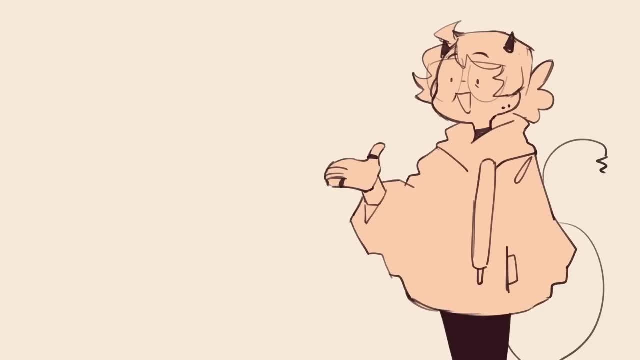 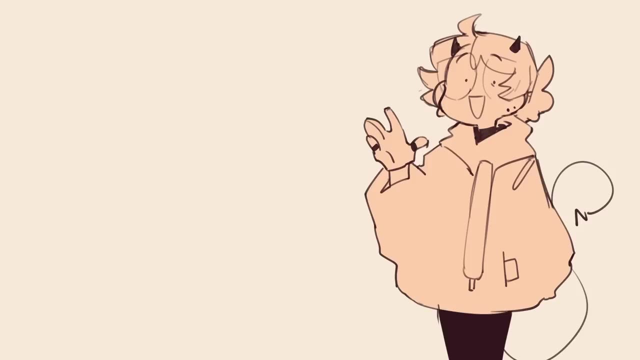 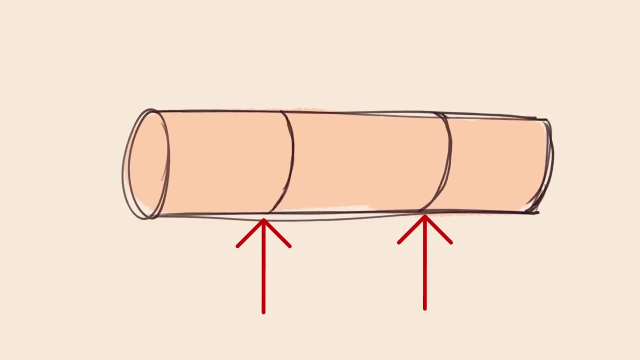 a lot closer to the camera. A good practice is to draw a bunch of shapes in wacky, creative angles. so let's move on to the next thing that will really help with perspective. it's something called the rubber bands. rubber band is a line that wraps around a shape. you can think of it. 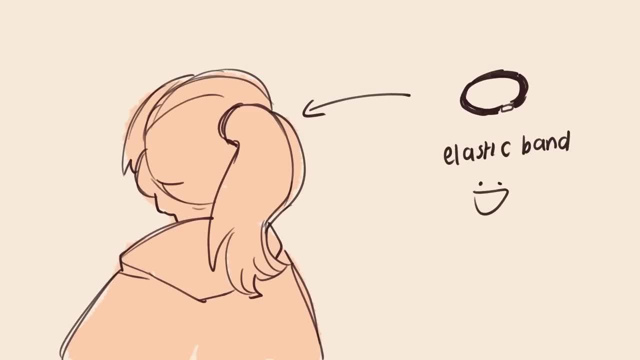 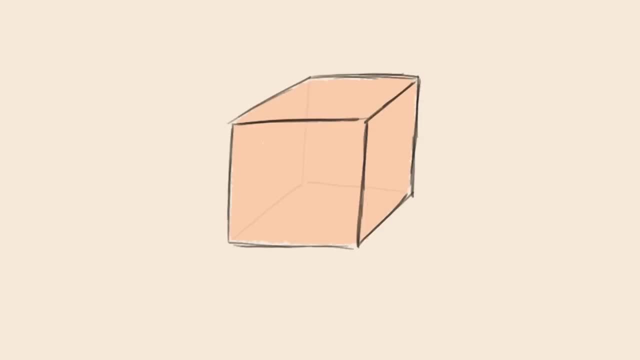 almost like an elastic band that wraps around the width of a shape. rubber bands are helpful to be able to keep track of the width, length and center of the shape. here's a square where i have added the rubber bands. so here's the length, here's the width and here is the center. you can almost 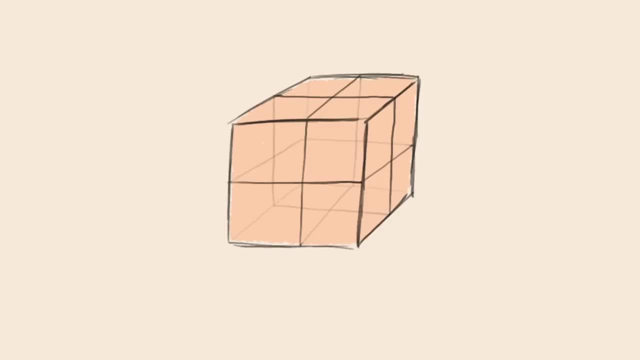 imagine it where you've put the rubber band. if you cut that shape in half and you look at it, you'll be able to see what kind of shape the rubber band has kept, if you know what a single line circle looks like. so just a circle like this, but from different angles, it'll help you determine. 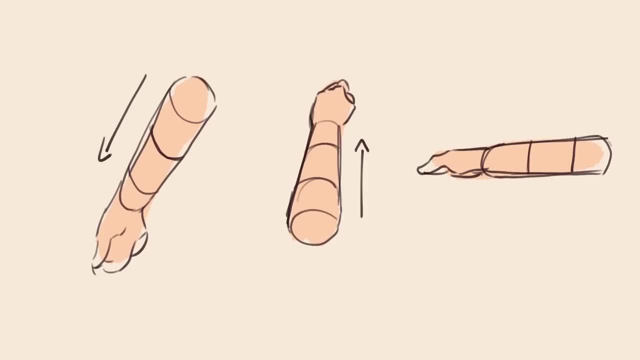 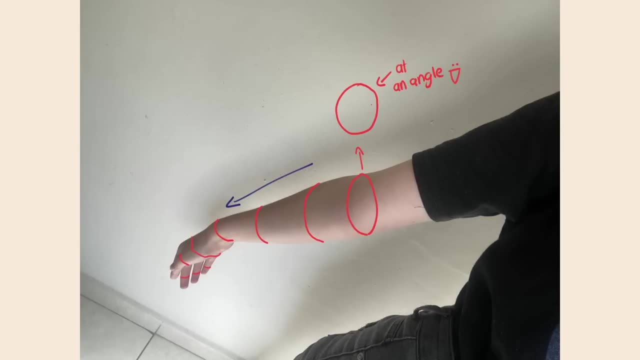 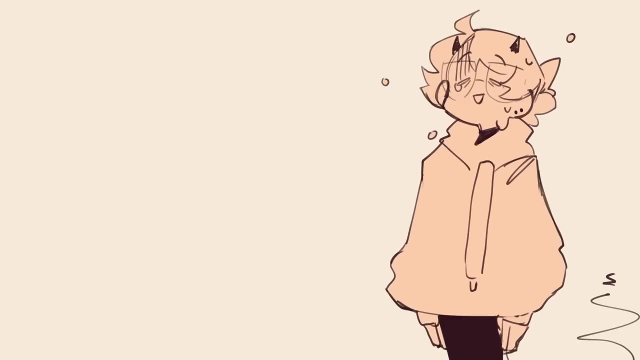 where the where the shape is going and in what like direction the shape is going. here's an example. as you can tell, the circle, like angle, changes the more my arm moves. so if my arm moves downwards, the circle is now angled like this, but if i move it towards the camera, it's kind of angled like this. now, if you learn this, this will. 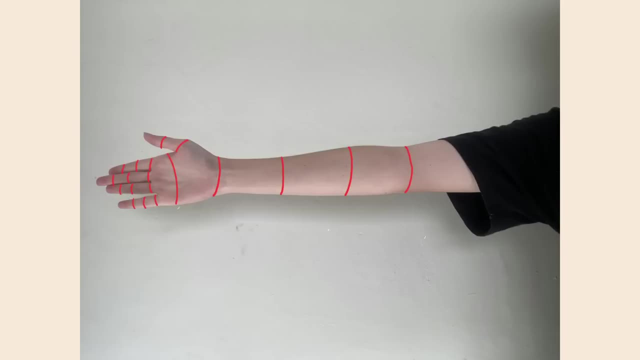 help when you're drawing perspective. i have two rubber bands here on my arm. the space between the rubber bands won't change. from the side view they're equally apart. but the moment i start moving my arm towards the viewer, the space between the two rubber bands will get smaller and smaller. 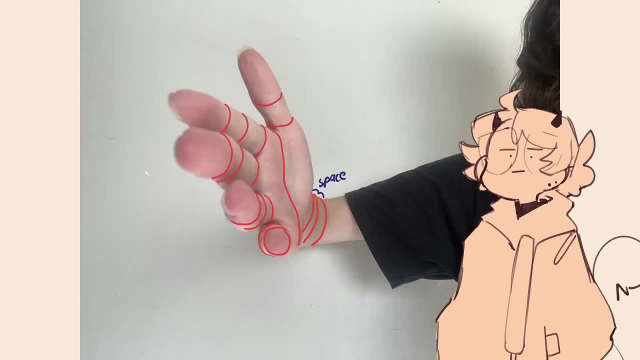 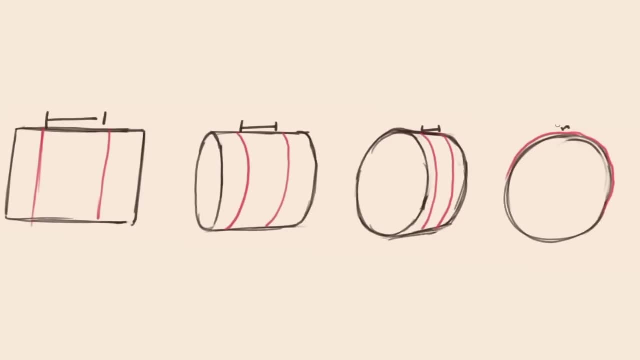 but you will still see the two rubber bands on my arm because, like they won't just disappear for no reason, this is called foreshortening. you want to make sure you can fit the right amount of rubber bands on the shape you've added, from all different angles. i promise this makes perspective so much. 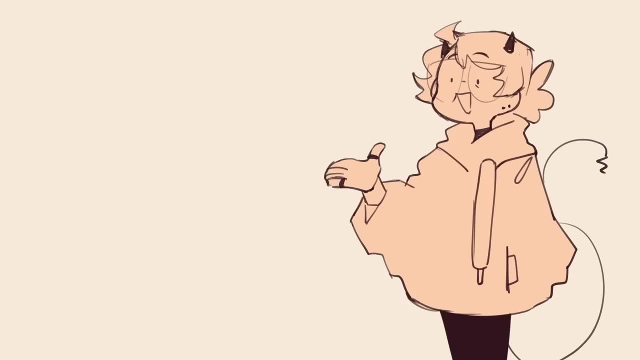 easier, especially angling body parts and making sure the body parts kind of stay the same proportions as they're meant to be so they don't kind of look wacky. for shortening, it is important to keep in mind the width of the rubber band and the length of the rubber band so that when you're 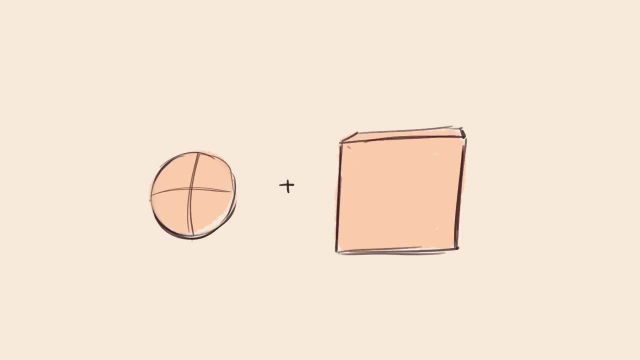 drawing, you don't have to worry about getting the right size, so it's a great way to keep the right size, even if you're drawing. you just have to keep the right size and the width of the rubber band and the size of an object. if an object behind is bigger and the object in the front is smaller, you 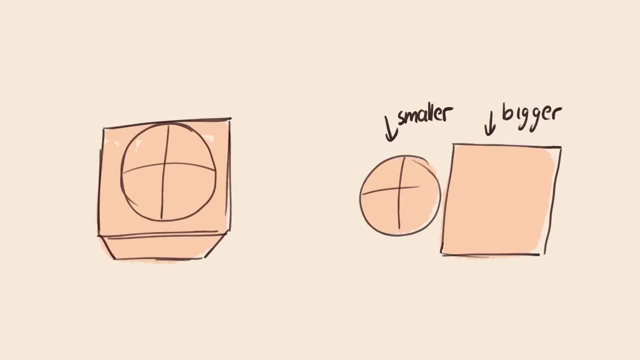 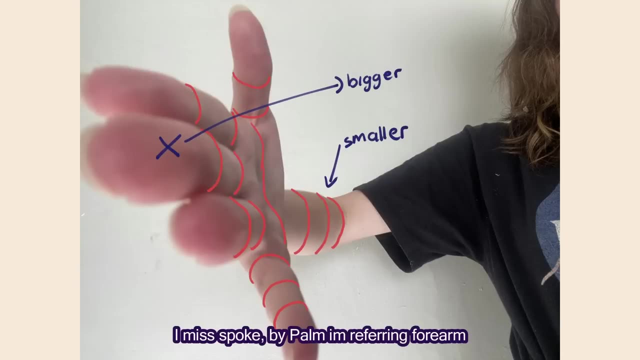 will see. you will see the object behind through the, the one that's in the front, because it's a lot bigger and it will show here. for example, my palm is obviously a little bigger than my fingers, so even though my fingers are in front of my palm, you will still see my palm, but you can also see my 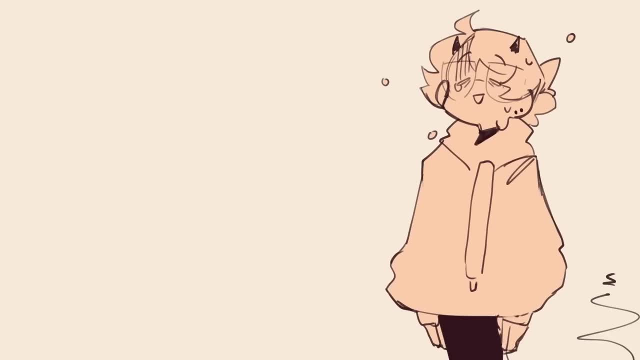 fingers. it's just because it's bigger, but because my palm is a little bit bigger than my forearm, you won't see that much of my arm, much of my forearm. so you really have to like learn the shapes and the sizes of anatomy and like which parts are bigger and which parts are smaller. so this is also where rubber bands can. 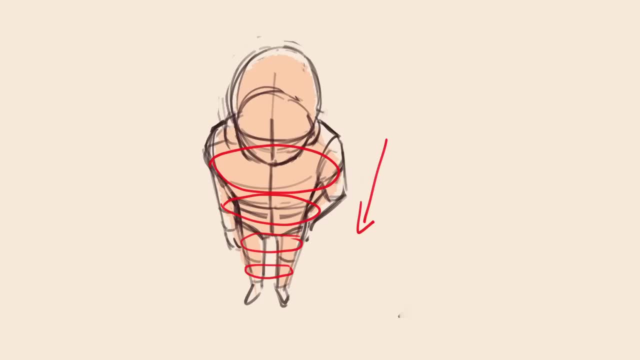 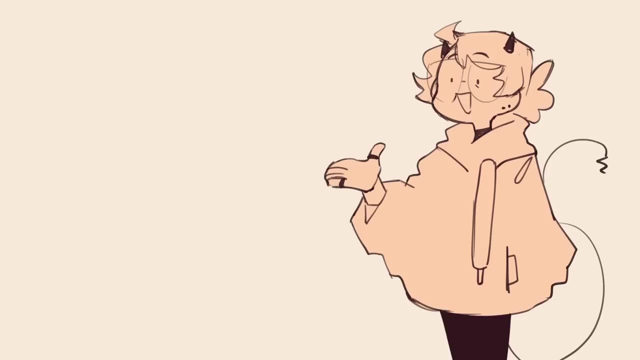 come in handy because you can keep track of, like how big or how many rubber bands should be on the body part, and remember the object that is further away will be smaller than the object closer to the viewer. now let's get down to drawing figures in perspective. this seems a little intimidating at. 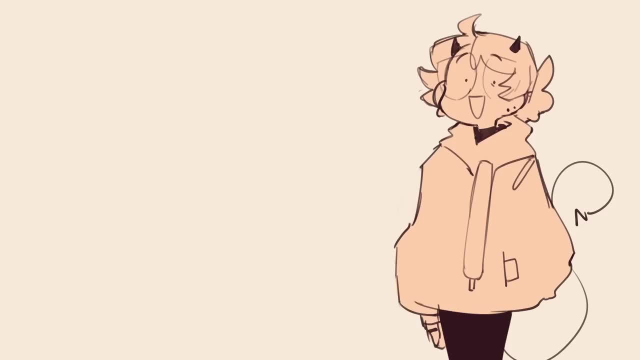 first. but if you know some of the basics of anatomy you can learn this pretty easily. first thing is to know the shape of anatomy. i have a video of how i made anatomy into simple shapes, if you're interested, linked in the description, or you can figure it out on your own and break. 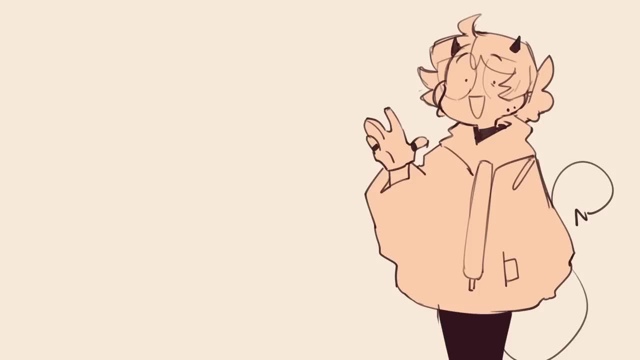 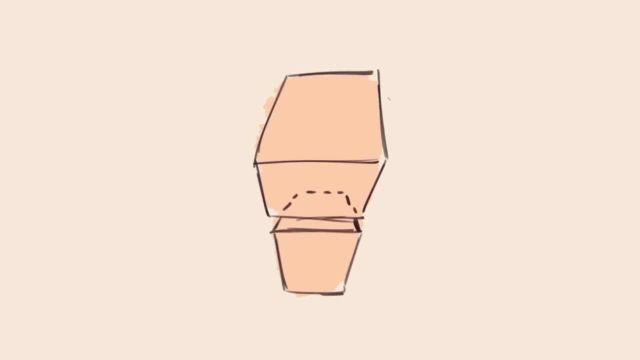 the anatomy down into shapes that you understand. but just basically having them in shapes is important, but the important thing is just being able to put them into shapes so you'll be able to stack and figure out where everything should be going when you start drawing it. for example, here are an arm and here are the shapes i used to define them. i've added rubber bands to. 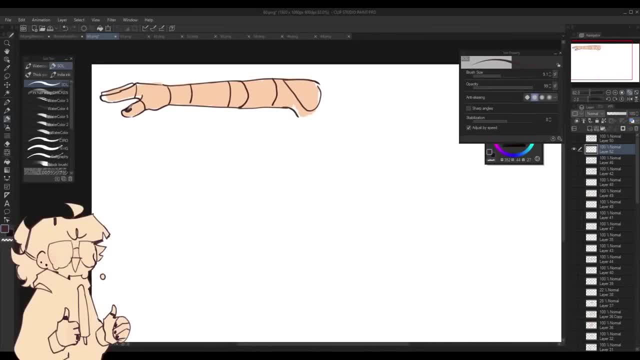 the arm right. i will keep the diagram to the side so it's easier to see which shapes should come first. so i want to put the the fingers and hands closer to the viewer. so it'll be this shape first, and then this shape, and then this shape and then the shoulders. so i'm just gonna go down in a line. 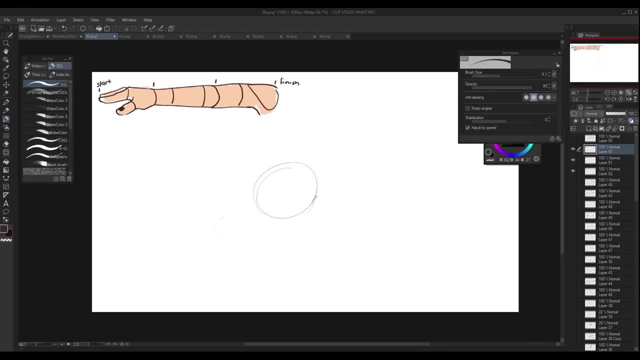 like this: make sure you're keeping the rubber bands there even when you're drawing like the perspective. so here i will start drawing the finger. i know what the finger looks like. i know what the cylinder looks like from all shapes and sizes, so just drawing this is a lot easier then. 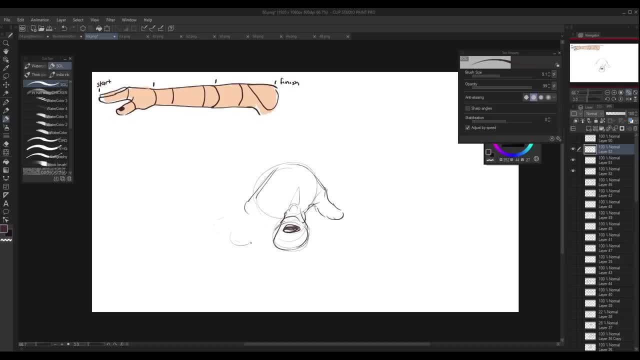 i'll move to the palm, then i'll do the forearm and then the upper arm and then the shoulder. you can probably notice that in some spots i draw the rubber band first. this is because it's easier to plan, so i would draw circles in the direction that the. you know the shape is going like i did. 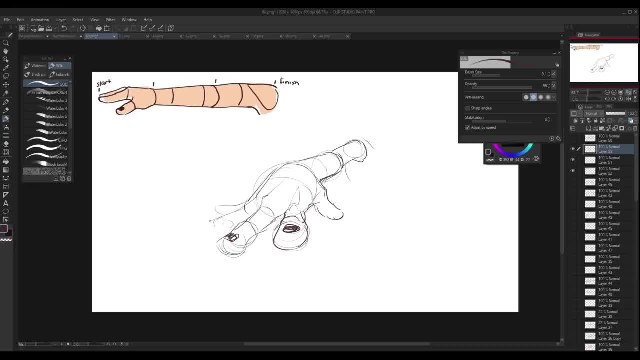 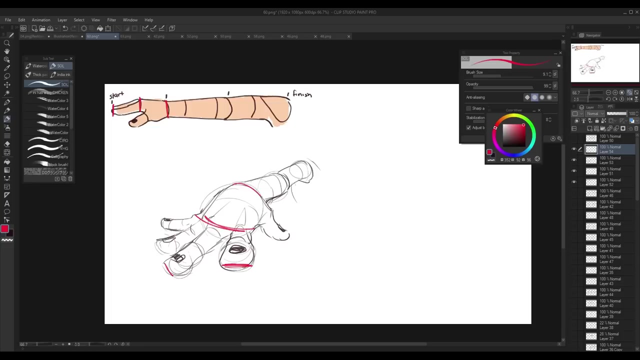 with the arm and then the fingers. uh, yeah, i i feel like this just makes it a lot easier to plan out where everything is going and, uh, like the angle that the thing is supposed to be in, it's basically like stacking shapes from front to back. now you can do this reversed as well, if you want to do it from the shoulder. 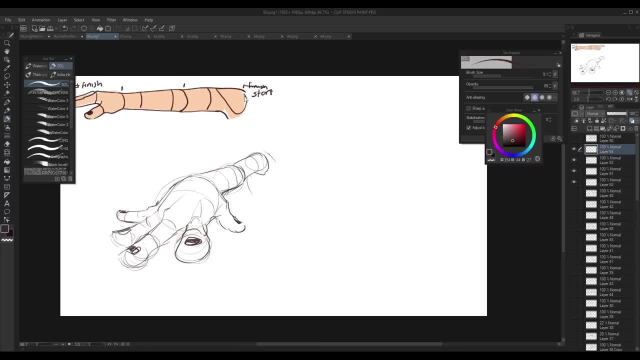 it'll just be reversed, so your starting point would be here instead. so shoulder, upper arm, forearm and then the hand. again, it's just keeping track of, like, where the objects would be and then the size of the object so you can see with the other angle. i drew the hand a lot smaller because 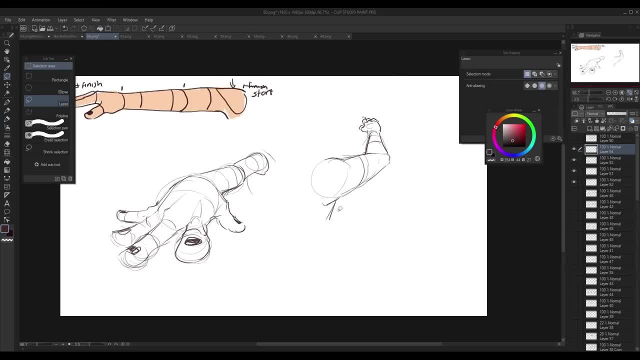 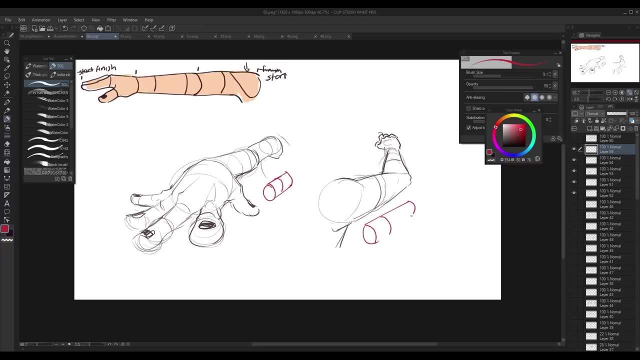 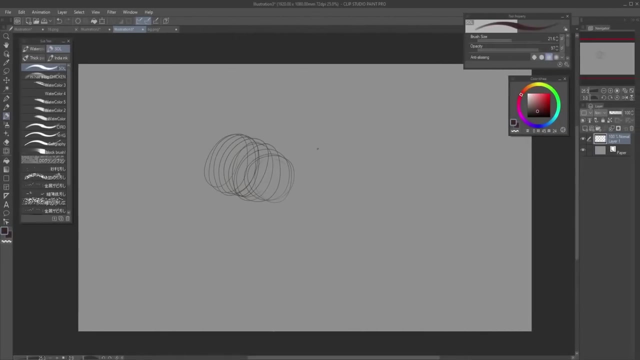 it's in the background, it's a lot further from the viewer, and here i'm just showing you the shapes i use. as you can tell, they're just cylinders, so if you learn to draw cylinders, you can basically draw almost anything. another method to do with rubber bands is: 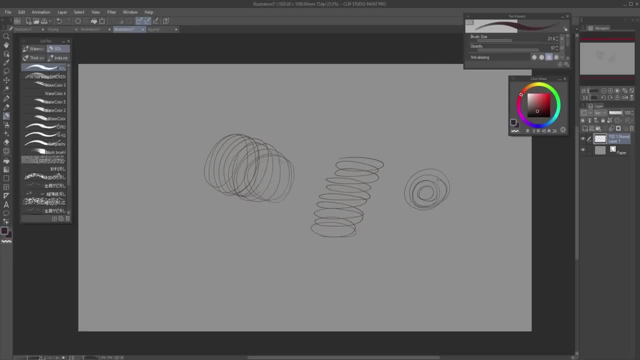 something called spiraling. this is, instead of drawing the actual shape first, you will instead draw spirals in the direction the shape is going. you can think of it as a spiral, and then you can think of these spirals as rubber bands, but they're all connected together, so you use the spiral method. 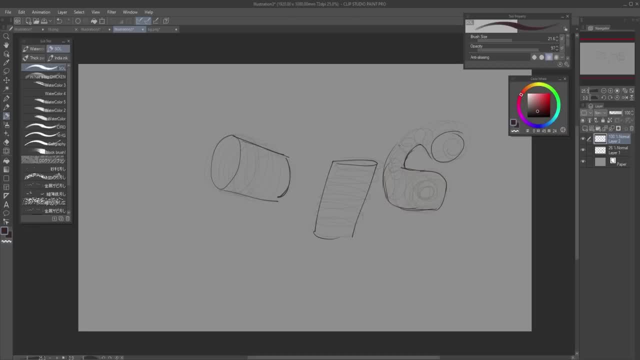 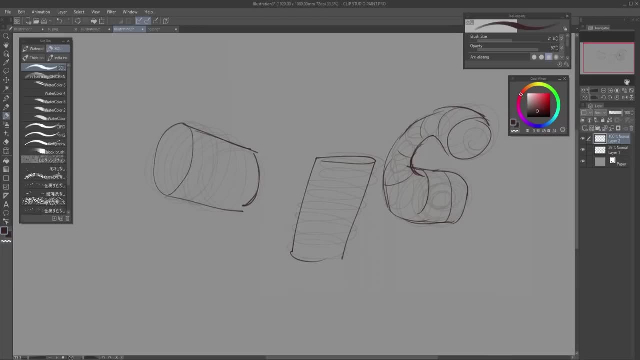 to plan out in what direction or perspective the body part or shape will be in. the spiral method can be very useful to draw for foreshortening, since you can make the spirals go from bigger to smaller, which can lead to some pretty neat and interesting perspective drawings like in this. 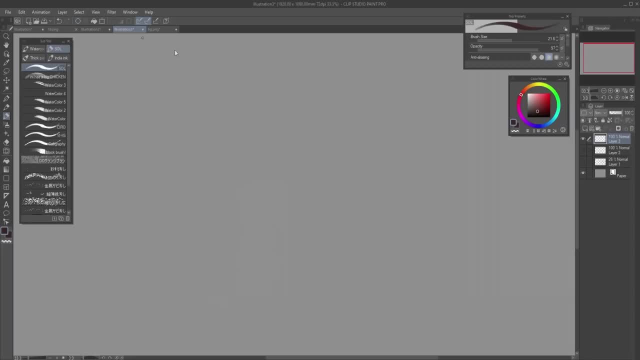 drawing, i started the spirals from bigger foe's feet and then made them smaller towards his head, because that's further in the background and that helps you plan out the body and in which direction you're going to go. it's also very useful for width and overall shape, since the spiral will be the same size as the rubber bands. 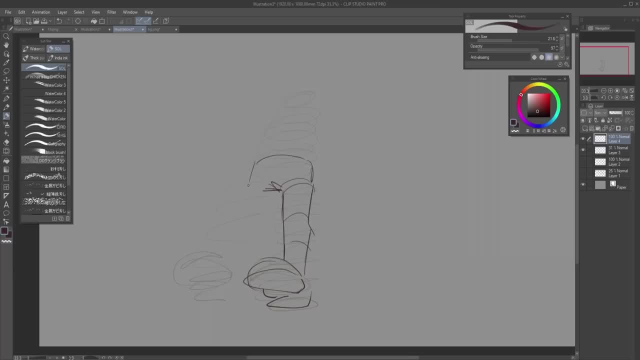 would portray- just think of it- as more aggressive rubber bands like your arms. i just made this to show you the width, length and angle of his arm, and then i just made the layer lighter and then i drew over it because it was like a reference for me. 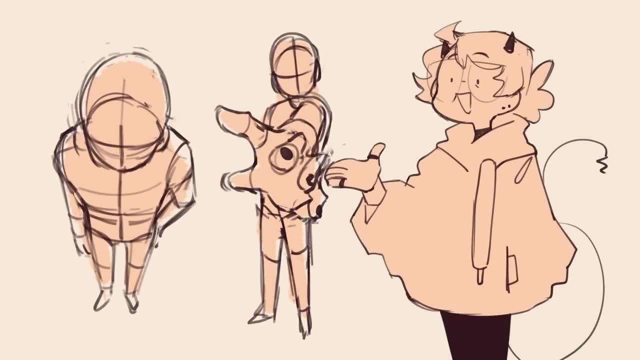 now, once you're comfortable with anatomy, you can do this with the whole body. this requires a lot of thought and to keep track of all the shapes and the replacements, every shape needs to be taken in your drawing style. and to keep track of all the shapes and the replacements, every shape needs to be taken in your drawing style. 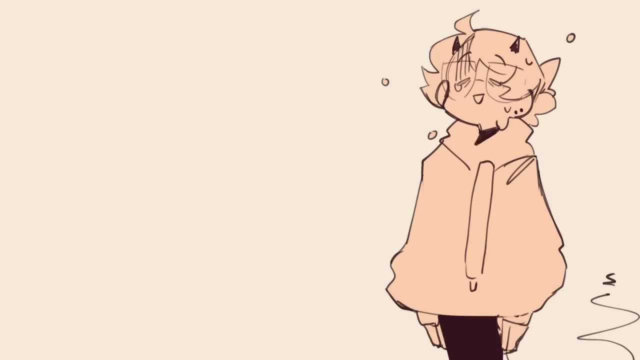 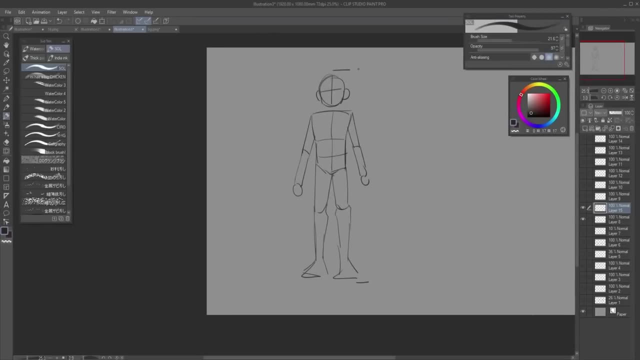 into consideration and aware there'll be Again. make sure you're keeping track of the rubber bands and making sure that the width you're thinking about like every body part, as a full shape, not just as like a line. So from top view, you'll start from the head and torso. 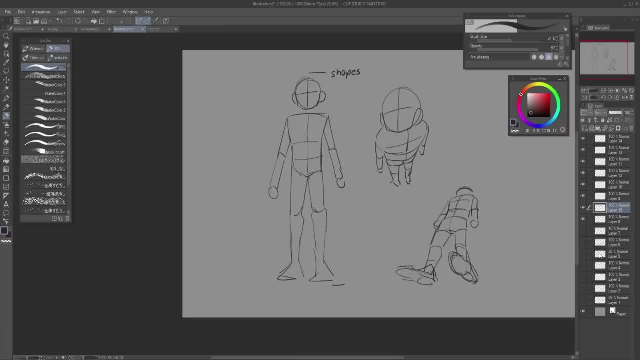 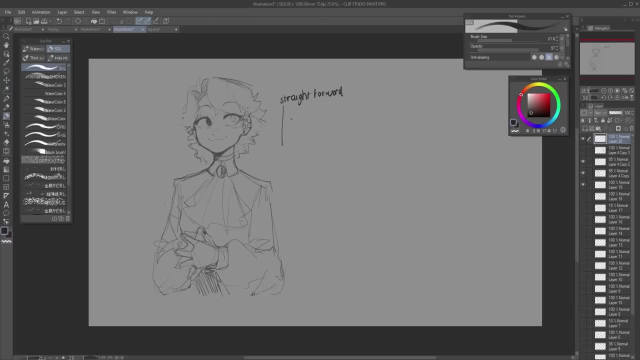 arms, crotch, legs and then feet, And then you can do the opposite as well, like I did over here. Even adding just like a little bit of perspective to a piece can make it look a lot more interesting and doesn't have to be this tricky. 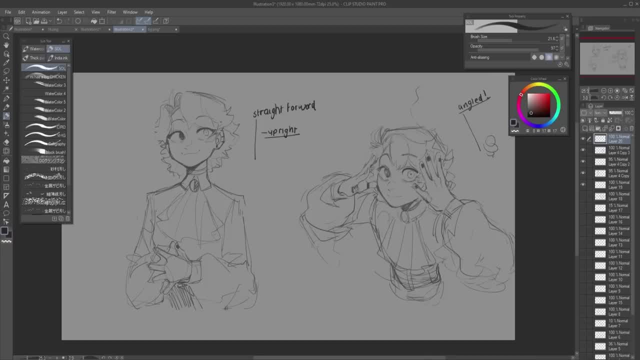 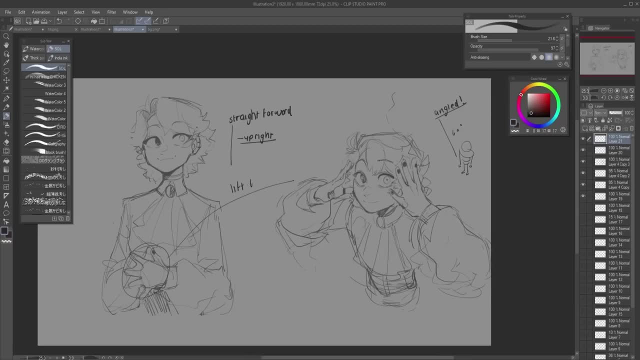 You can just lift an arm towards the viewer or you can have an arm further back from the viewer. Just adding just a little bit here and there, it really helps the piece come to life. Remember, it's okay if it looks goofy at first. 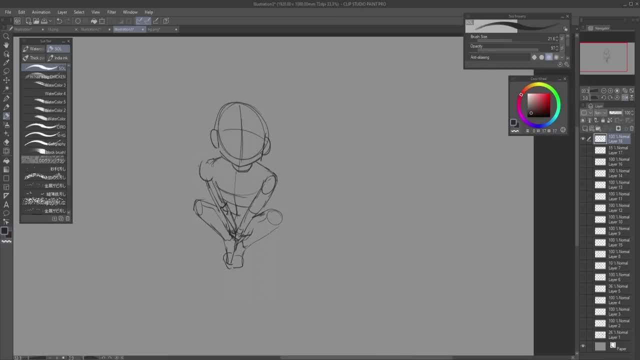 especially if you're just starting out. I think that's the funnest part about learning perspective is there's not much rules. It kinda, kinda, kinda messed up because you know it's perspective. it's goofy, So just have fun with it. 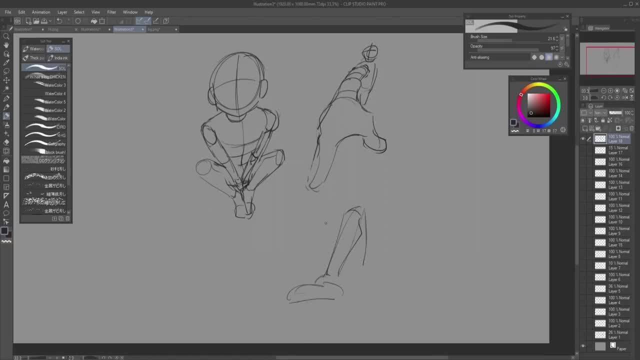 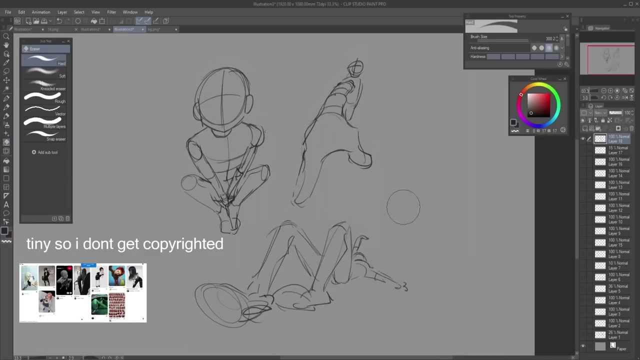 Just try drawing your figures like that And you know, after a while you'll start getting better and better and better and it'll become a lot easier. So I now have a Pinterest where I save references and study materials. So I have an album for pictures in perspective.